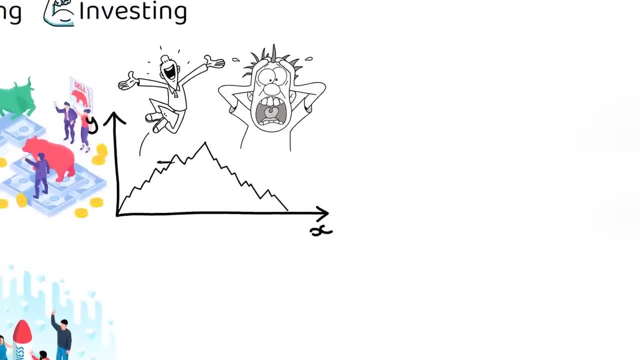 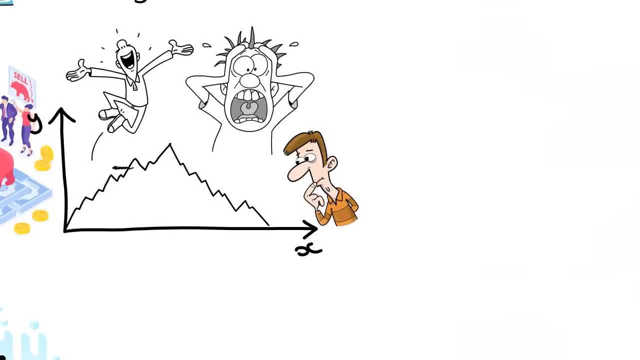 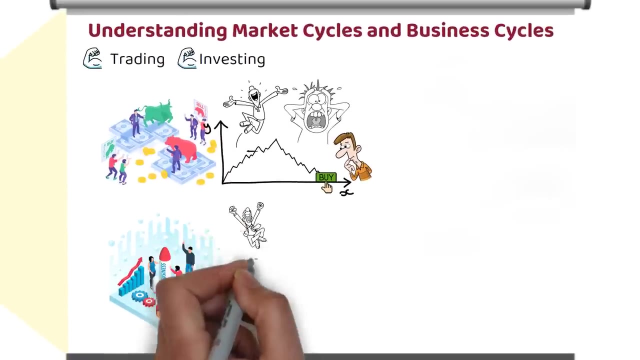 of markets and businesses. While the emotions of humans are busy creating cycles, there are less emotional, smart humans at the other end of the spectrum who are relatively unperturbed by these extremes and wait for such overreactions to play out. Because markets are driven by underlying business performance. it's only natural for naive 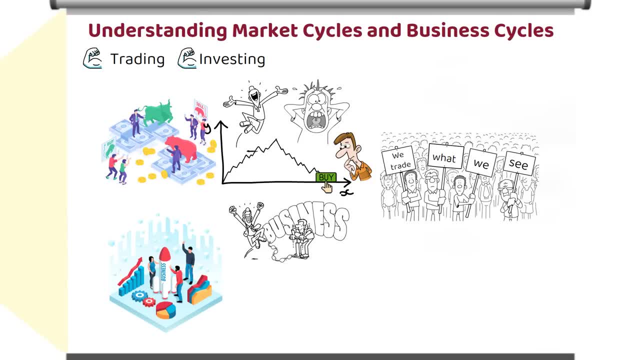 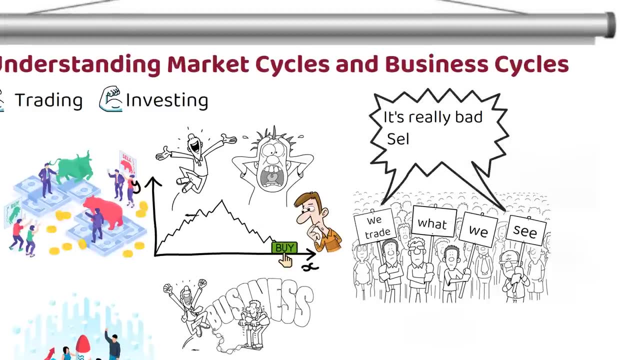 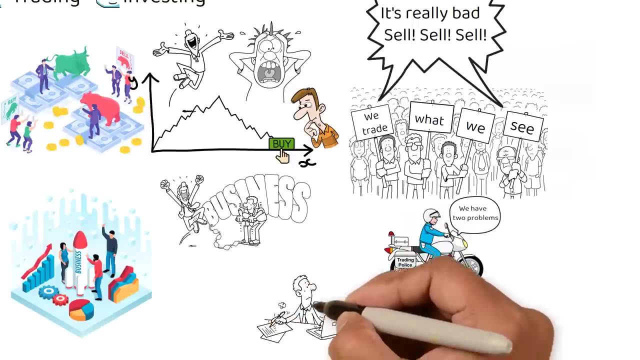 traders to place their trades based on the current economic performance. This leads to new traders becoming bulls when the economic data is at its strongest, whilst becoming bears when the data is all red. There are two problems with that approach to the markets. The economic data is a lagging indicator of what the economy is really doing. The data 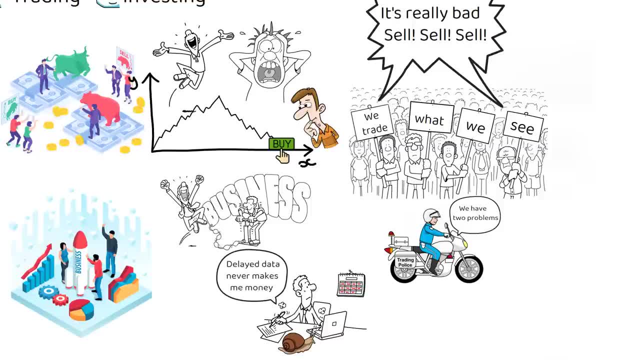 always shows the past performance and therefore isn't actionable in real time. Also, markets always follow a forward-looking mechanism. They don't go down when the economy is in bad shape. Instead, they go down when the market participants foresee the economy to be in. 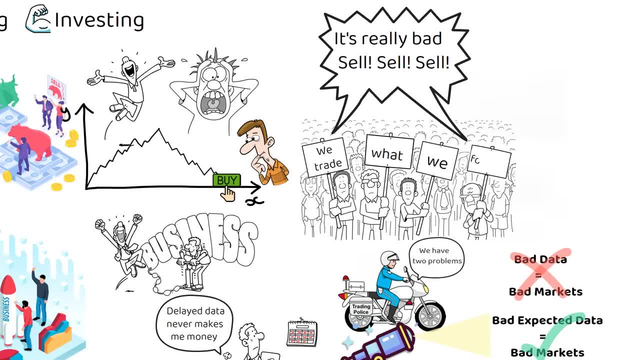 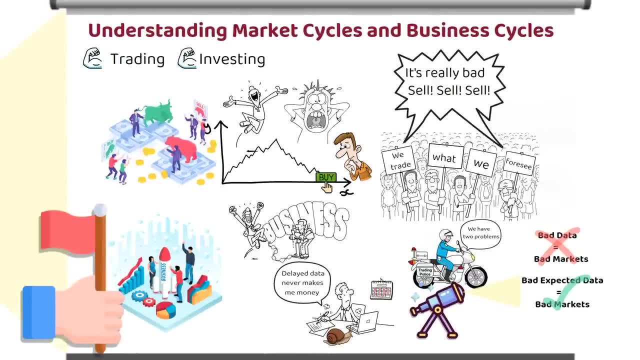 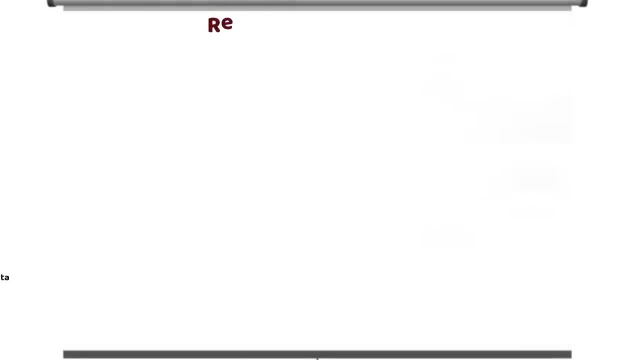 bad shape in the near future. The markets always see the best and worst before the economy sees it. Therefore, you must be aware of the leading nature of the market to trade well and trade profitably. Let's understand how the link between business and markets have played out in the past cycles. 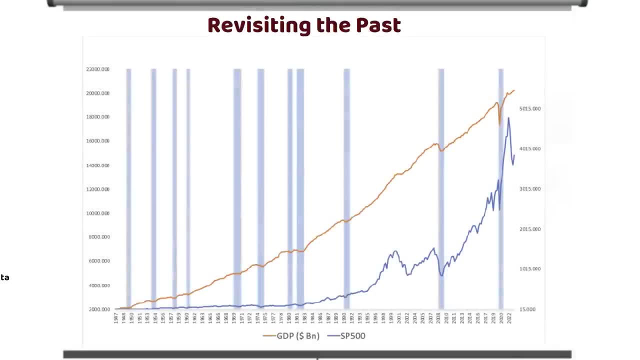 Here's a chart showing the performance of the economy and the S&P 500 over a 75-year period, from 1947 to 2023.. The shaded areas in the chart show 11 recessions and slowdowns in the past 75 years. The chart: 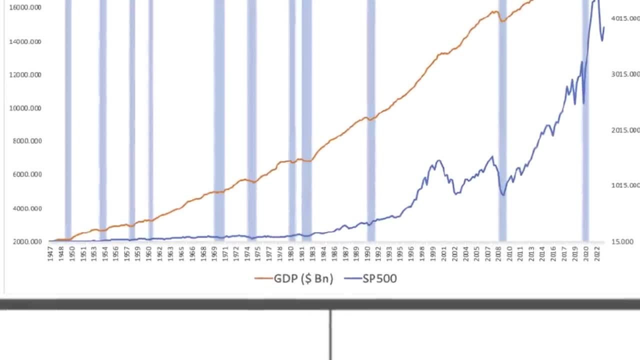 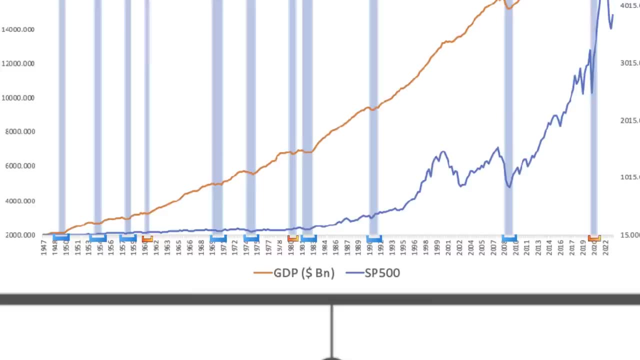 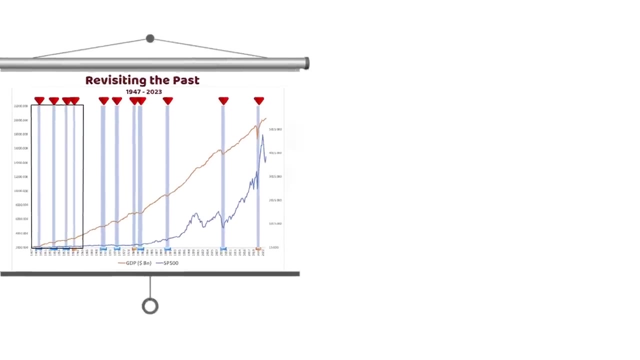 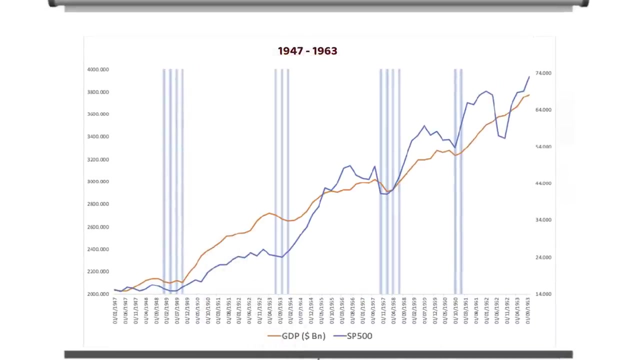 and the trendsico tag are linked to…. It's also the case that S&P 500 dropped to 20% in 2016.. 44% – Not that many people do- hot markets in general, whereas 5% of the market lost goods to their competitors following llama debt recessions. 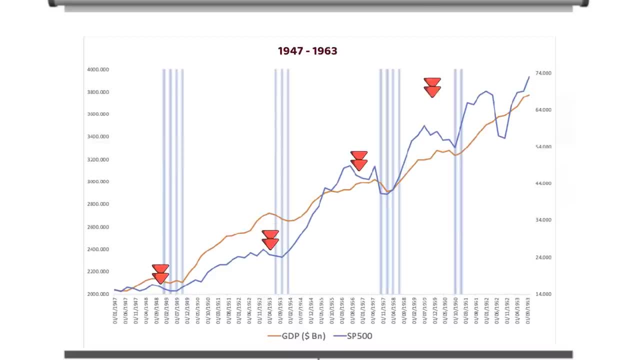 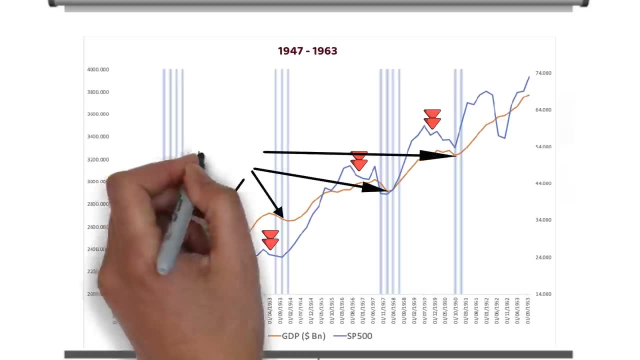 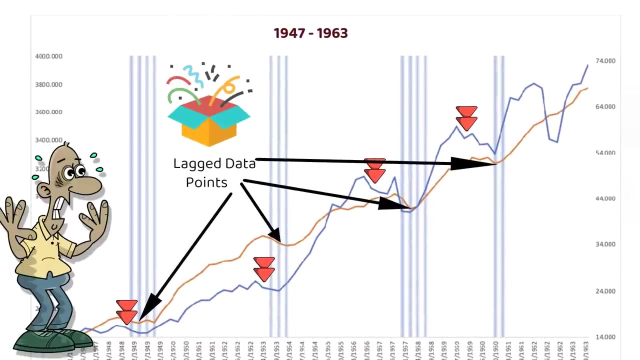 �uets before the recession settled in, The GDP data comes with at least a month's lag and by the time the GDP data came out, the index had already reacted to the data, Unless the data throws in a significant surprise. the index generally does not react to the GDP news when it finally comes out. 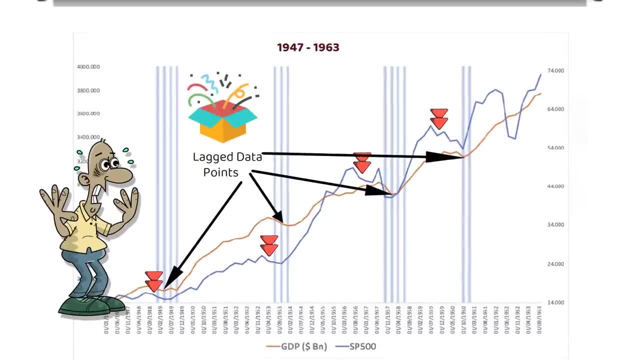 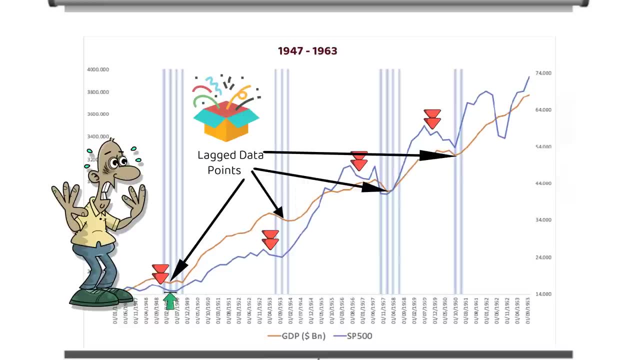 Another key point to note here is how the market index behaves during a recession and afterwards. Most times the market bottoms before the economy bottoms. It was very clear in 1949 and 1953 and not so clear in 1957 and the 1961 cycles, when the market bottom coincided with an economy bottom. 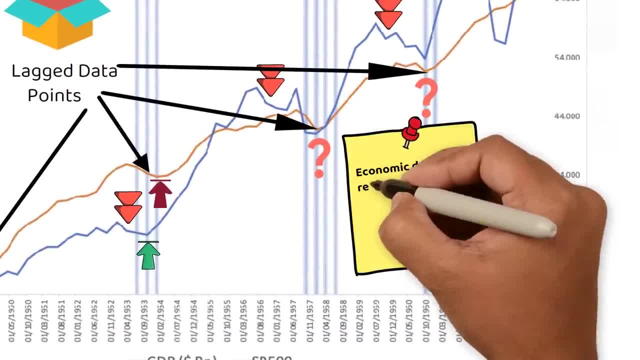 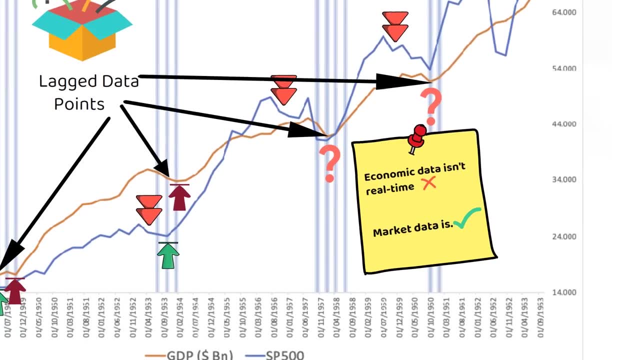 However, another point to note here is that the economic data is not real-time data, while the market data is real-time. Therefore, by the time the economic data is not real-time, it is not real-time. Therefore, by the time the economic data gets out and the economic bottom is clear, the market has already marked a 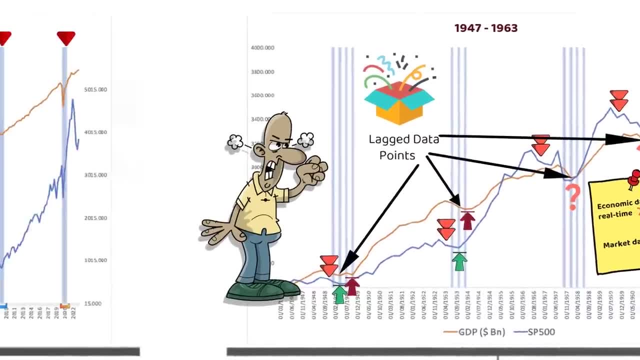 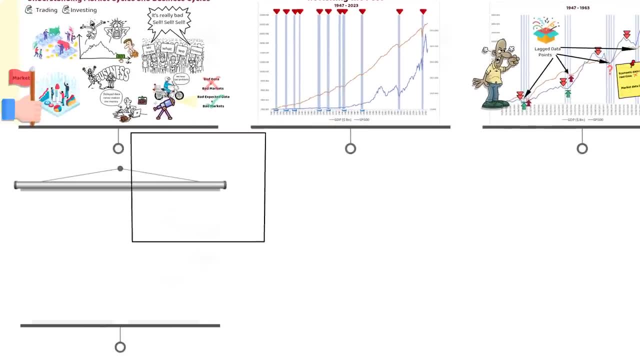 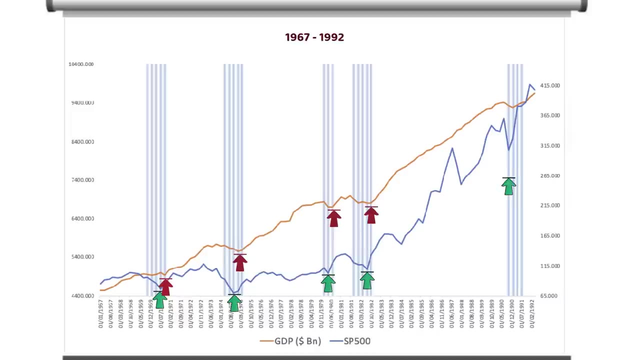 bottom and moved on. Let's look at another period, from 1967 to 1992.. Here also, the market bottoms before the economy and took to new highs much before the economy. As the governments and central banks become more responsive to these cycles, the 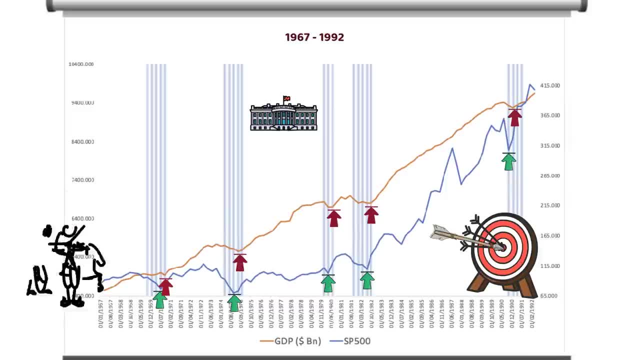 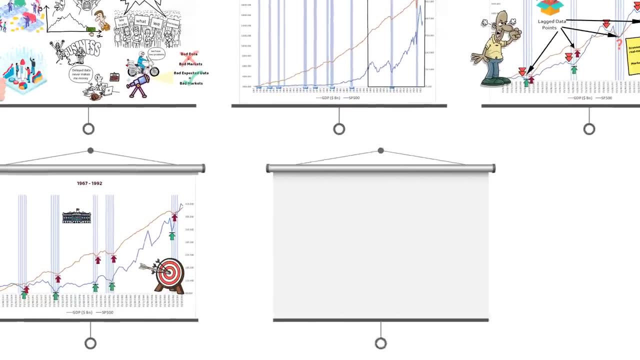 market has become more efficient over time, cementing the leading nature of the market. Let's look at the most recent period, from 1998 to 2023.. There are only two recessions in this period. If we remove the pandemic-induced recession, the current period would be the. 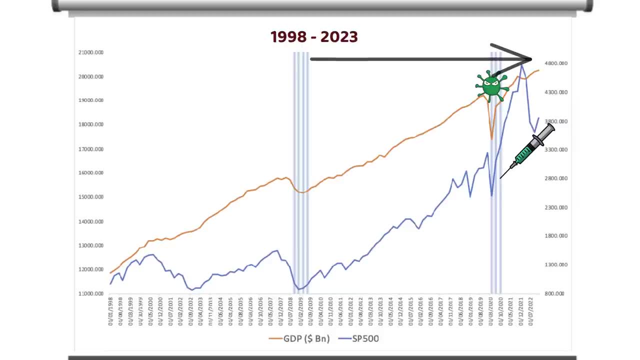 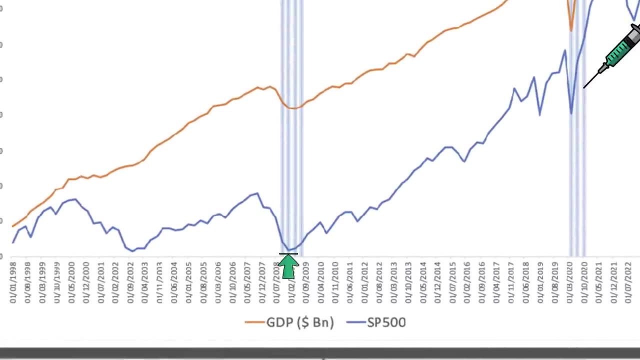 lengthiest period of economic expansion in the entire 75-year history. In the 2008-2009 economic recession, the market again bottomed before the economy, but took its own time to scale back to previous highs, due to a period marred by economic growth. 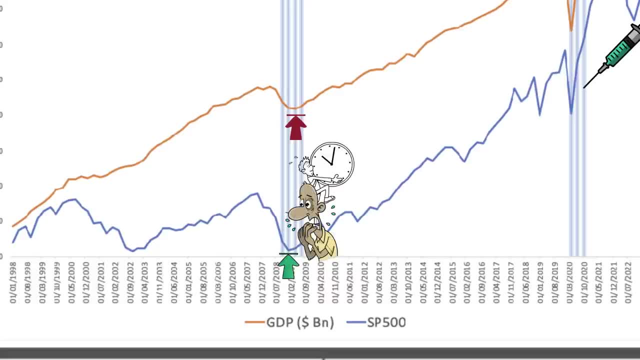 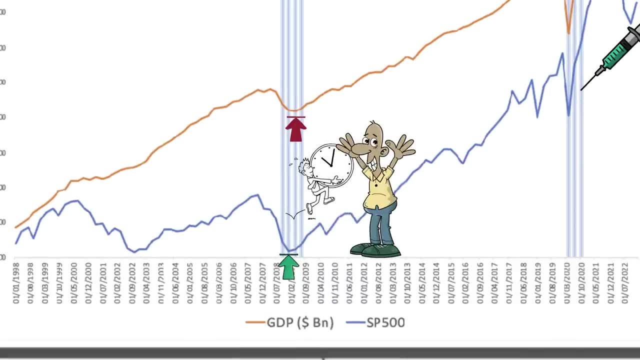 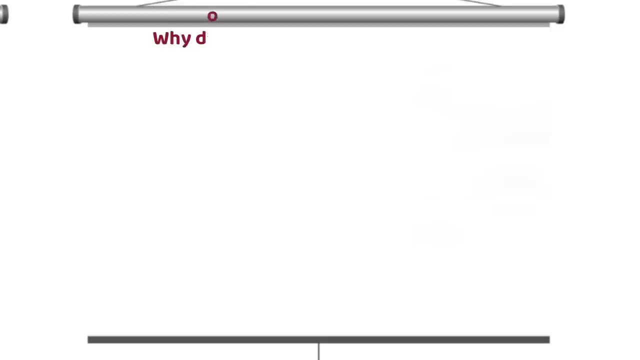 extreme risk aversion, given this was the most intense recession after the 1930s Great Depression. The market nevertheless shed the risk-off approach in the early 2010s and a new bull market began thereafter. You may wonder what leads to the market bottoming before the economy. 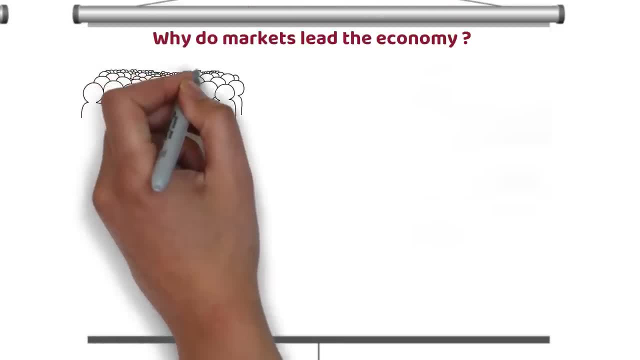 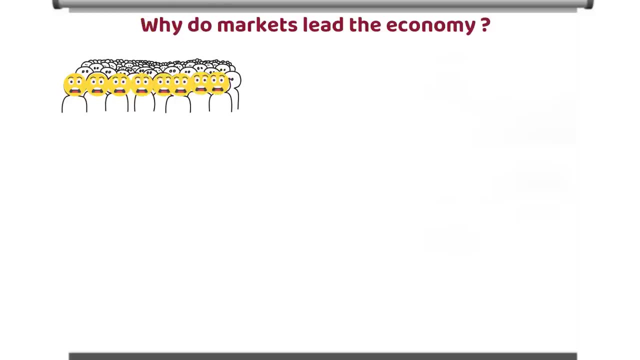 and scaling new highs before the economy hits new highs. The first explanation to this is that the market is full of scary beings who tend to react- and sometimes overreact- to anticipated bad data. This leads to market bottoms being formed in advance. When this fearful bunch of traders are selling, the baton is taken over by value investors.